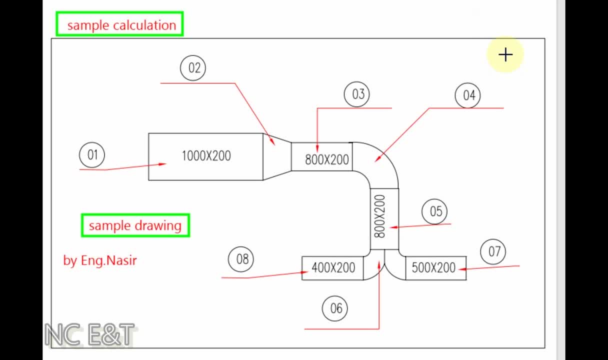 things are considered. now to learn the application of these engineering formulas to calculate the area of rectangular duct, we will make a sample exercise. your screen is showing a part plan of rectangular duct. to make more easy for the calculation of area for this rectangular duct, we have given the tag number to each piece of the duct. the tag number one is the rectangular. 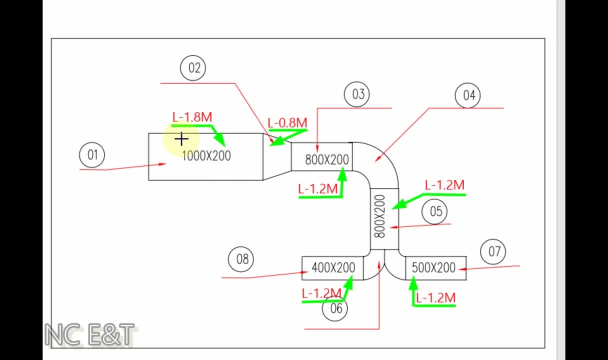 duct size: 1000 by 200, length, 1.8 meter. number two is the reducer between 1000 by 200 and 800 by 200. length is 0.8 meter. number three is the straight duct: 800 by 200, length, 1.2 meter. 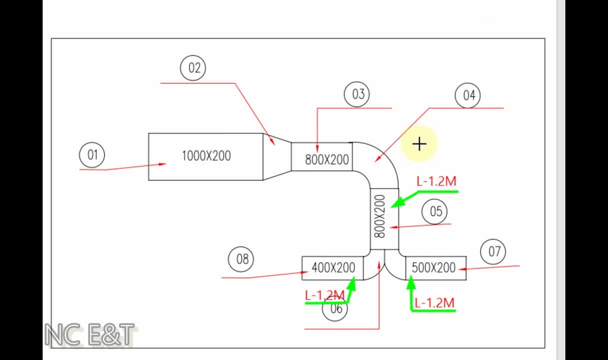 number four is the elbow: size: 800 by 200, and number five is the straight duct: size 800 by 200, length 1.2 meter. number six is the y branch: size: 800 by 200, 500 by 200, 400 by 200. number seven is the straight duct. 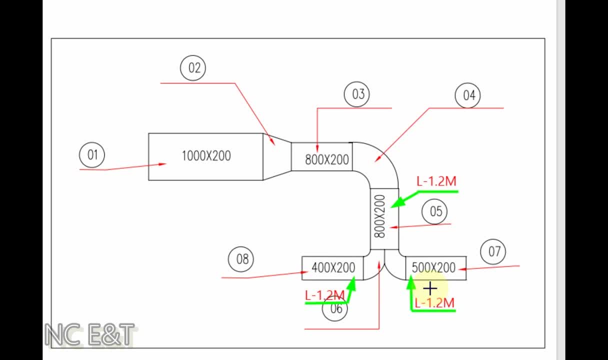 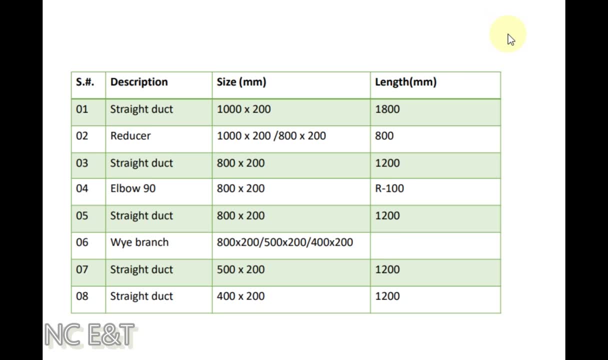 again: length: 1.2 meter. size: 500 by 200. and number eight is the straight duct: 400 by 200. length, 1.2 meter. for the purpose of area calculation we have tabulated the value of the shop drying. the first column is for the tag number, second column is for description and the third column is 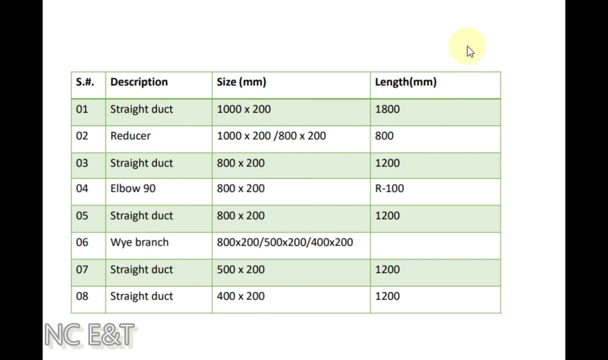 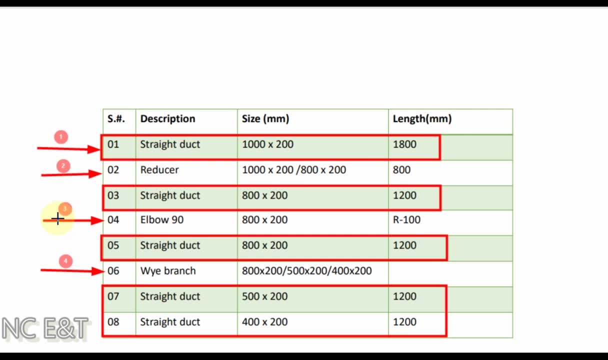 for the size of the duct and fourth column is showing the length of this duct. as you can see from the table, we have four types of duct. number one is straight duct, number two reducer, number three elbow and number four is the y brand. we will make the calculation one case from each type. 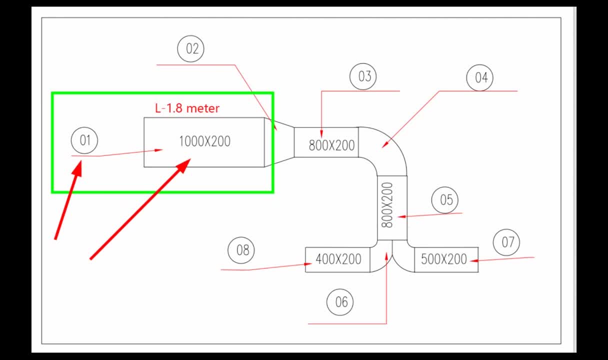 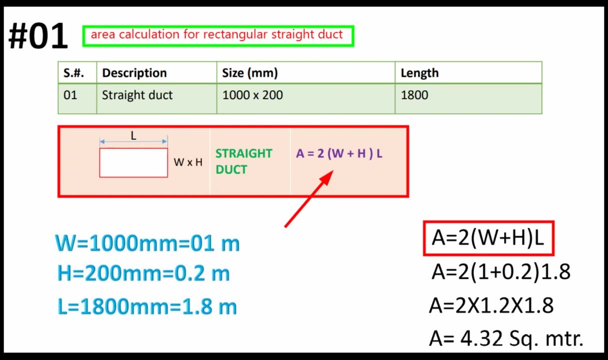 we will start our sample calculation from the item number one, that is, rectangular duct of size 1000 by 200, length 1.8 meter. as we have a straight duct of size 1000 by 200 mm and length 1800 mm, let us convert these dimension into meters with equal to 1000 mm, equal to one meter height. 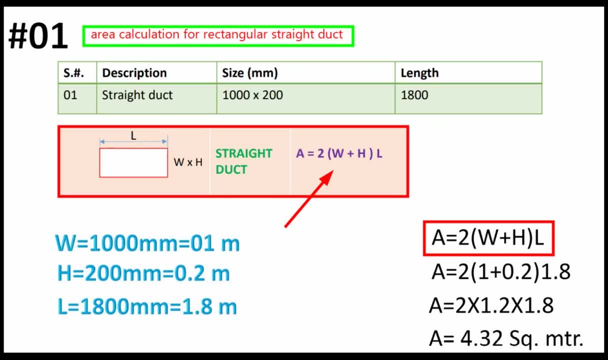 200 mm, equal to 0.2 meter, and length 1800 mm, equal to 1.8 meter. and we have the formula for the area calculation of a state duct: area equal to two times width, plus as multi VàN ch rhymes with "-2". 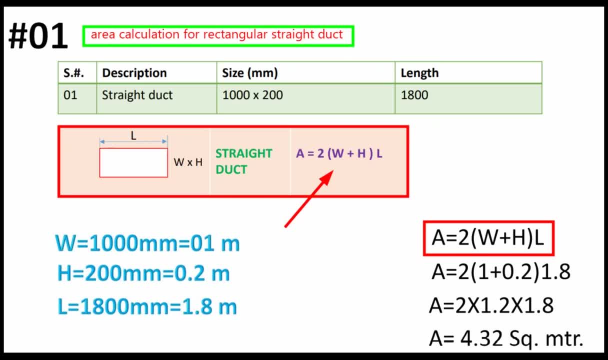 area equal to two times width plus H, aten Almost both of the área calculation delimited: dobrary cardícs: area equal two times width plus h. pentahciones equal to 2 times width plus h into l. When we will apply this value of width height. 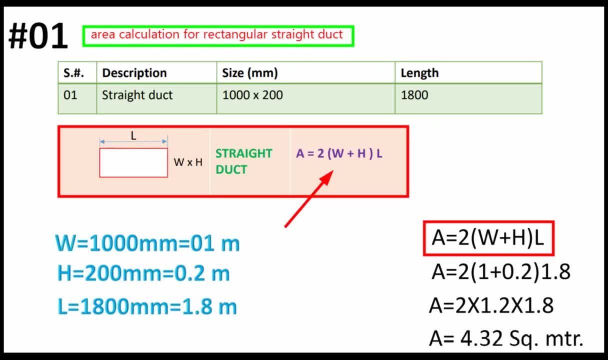 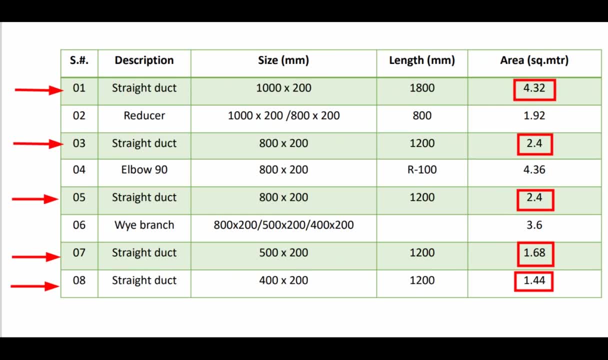 and length in this formula we will get a result: area equal to 4.32 square meter, As item number 3,, 5,, 7 and 8 are same like item number 1, straight ducts. so we can calculate. 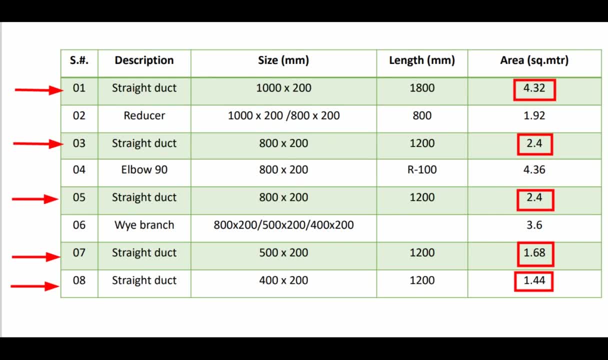 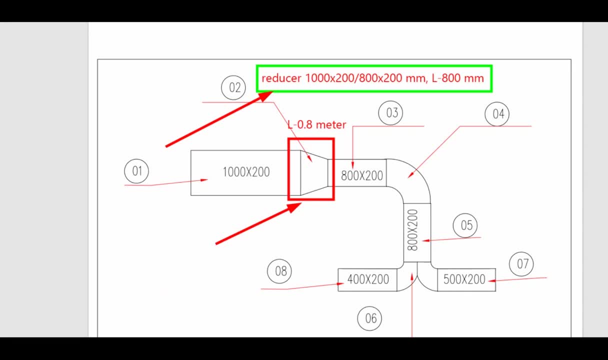 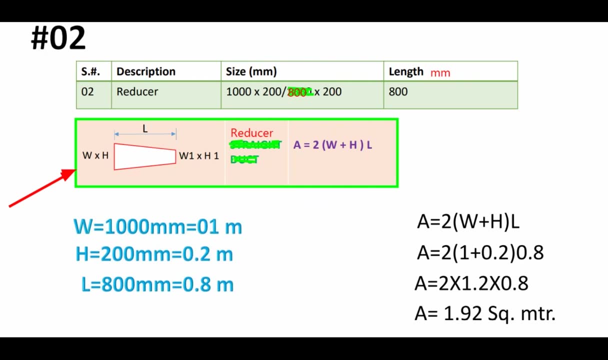 the area for this item in the same way as we have calculated for item number 1.. The second item is rectangular reducer having one side 1000 by 200 and another side 800 by 200, length of 800 mm. As second item, we have a rectangular reducer having size 1000. 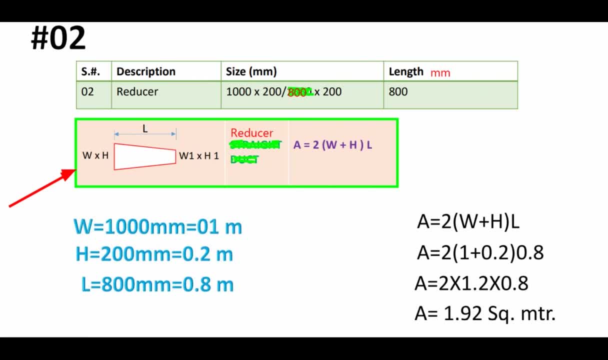 by 200 by 800 by 200, length, 800 mm And, as we know, the formula from the table for a reducer area equal to 2 times width plus h into l, where width and h is equal to 4.32 square. 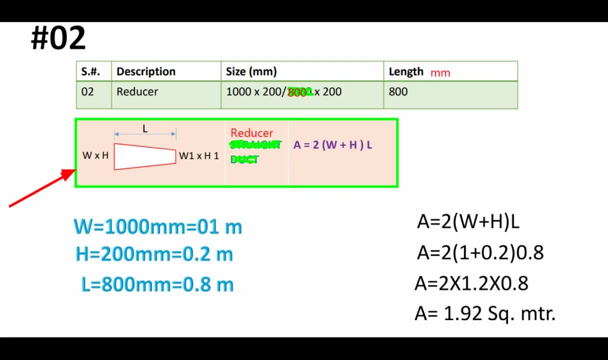 meter. This is the dimension for the largest side. Let us convert these values from millimeter to meter. Then width equal to 1000 meter will be 1 meter. H equal to 200 millimeter will be 0.2 meter. Length, 800 mm will be 0.8 meter. 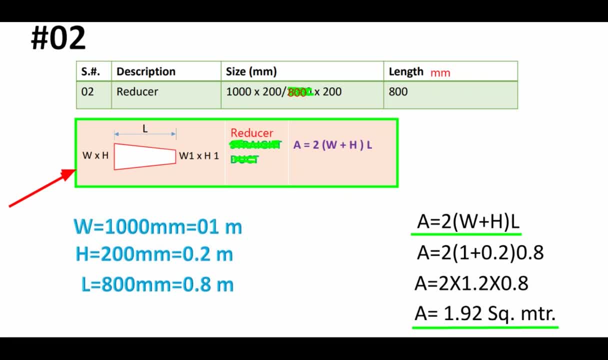 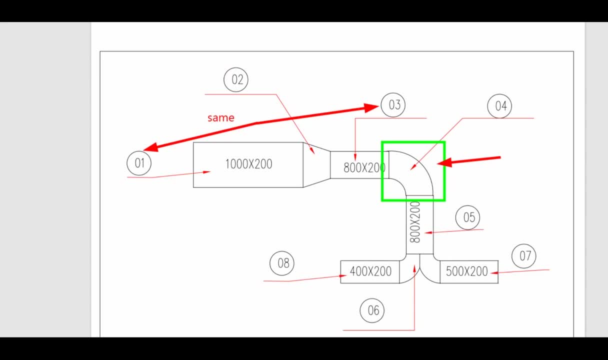 As we know, the area equal to 2 times width plus h into l. When we will apply this value in this formula, then we will get a result area equal to 1.92 square meter. Item number 3 is a rectangular dust, and its area can be calculated in the same way as: 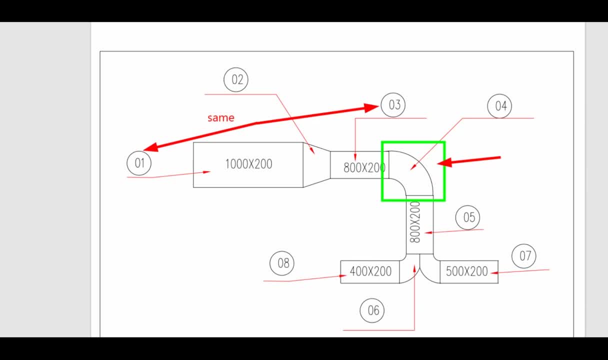 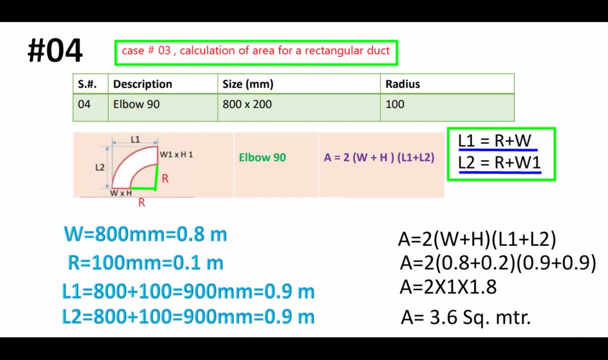 we have calculated item number 1.. Item number 4 is an elbow having dimension 800 by 200 mm. witch width and height are the dimension for the largest side and l 1 we can calculate from here. l 1 equals to width plus r and l 2 equals to width 1 plus 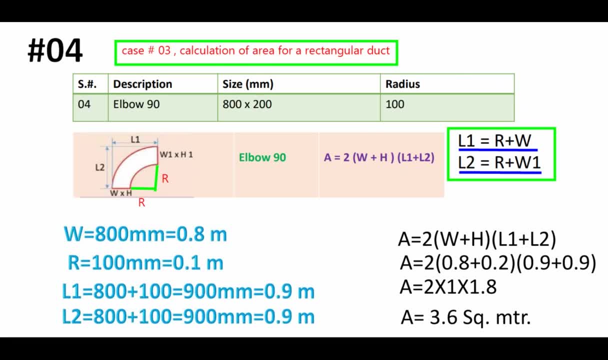 r. Let us convert these values from linear to dimensional value, intoant to continuous, We can find the acceleration and the speed. Now we can keep on evaluating. Let us start. the calculation of flex and torque Cont vector is measured by즈 h of le den's. This is V. 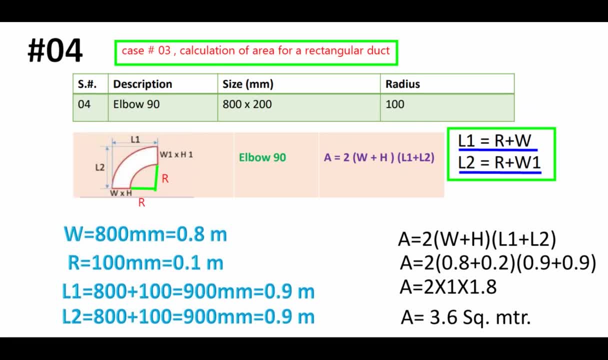 from mm to m, Width will be 800 mm will be 0.8 m. Radius, 100 mm will be 0.1 m. L1- we can calculate as 800 plus 100, equal to 900 mm, and it will be 0.9 m In the same way, L2. 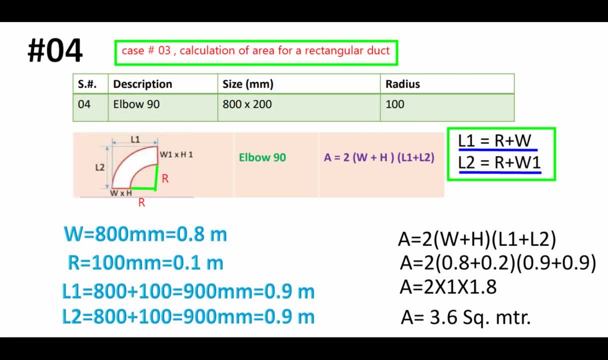 will be 800 plus 100 mm. 900 mm will be 0.9 m. When we will apply this value in the formula area equal to width plus h, into L1 plus L2, then we will get a result area equal to 3.6. 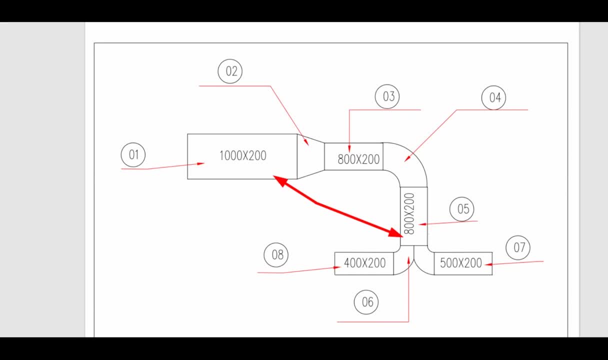 square meter. Again, item number 5 is a rectangular duct and the area can be calculated, same as like item number 1.. Item number 6 is a Y-branch having dimension one side 800 by 200 mm, the second side 500 by 200 mm and the third side 400 by 200 mm. 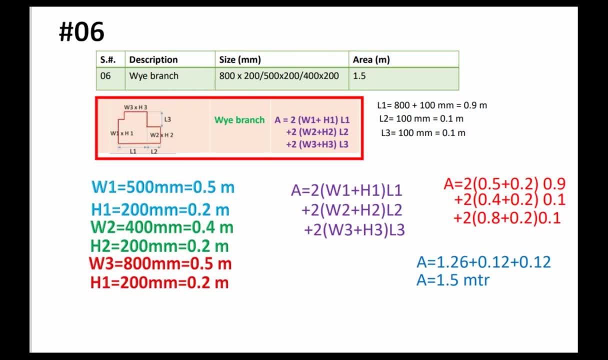 As we can see, the area is equal to width plus h into L1 plus L2. then we will get a result: area equal to 2 times width plus height 1 into L1, plus 2 times width 2 plus height 2 into L2, plus 2 times width 3 plus height 3 into L3.. Assuming radius for this Y-branch: 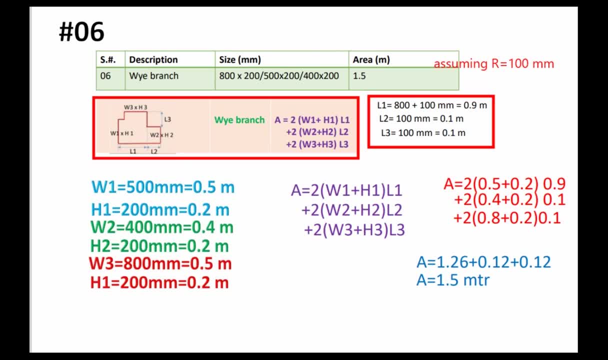 equal to 100 mm. then we can calculate the value for L1.. L1 will be equal to 800 plus 100 is equal to 900 mm and it will be 0.9 mm. L2 will be 100 mm and it will be 0.1 meter. L3 will be equal to 100 mm and equal to 0.1. 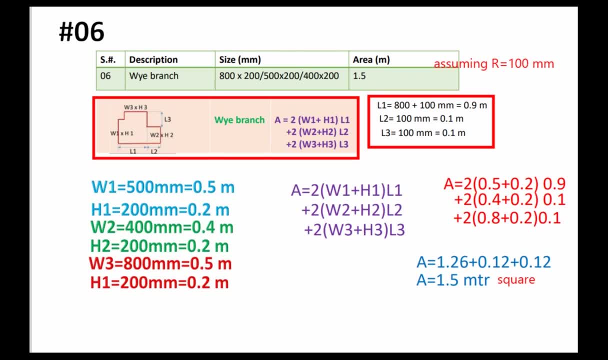 meter. Let us convert to rhyme these values from millimeter to meter. width 1 to 500 mm will be 0.5m. height 1 to 100 mm will be 0.2 m. width 2 to 400 mm will be 0.4 m. height 2: 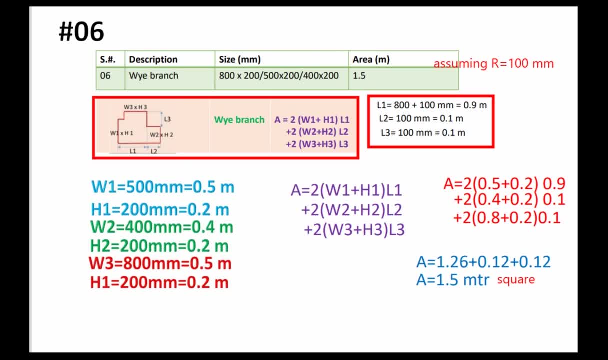 to 100 mm will be 0.2 m. width 3 to 800 mm will be 0.8 m. width 3 to 800 mm will be 0.6- 8 meter and height 1 200 mm will be 0.2 meter when we will apply this value to. 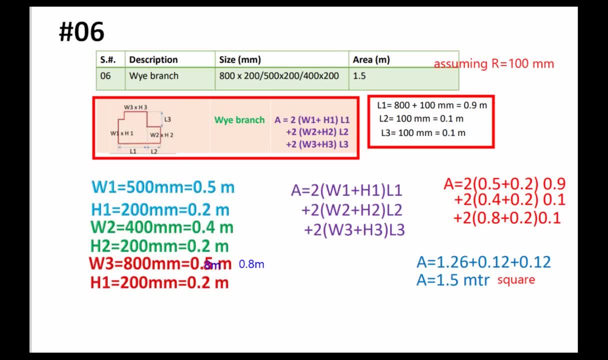 the formula area equal to 2 times with 1 plus H, 1 into L 1 plus 2 time W, with 2 plus height 2 into L 2, plus 2 times with 3, height 3 into L 3, then we will get a.